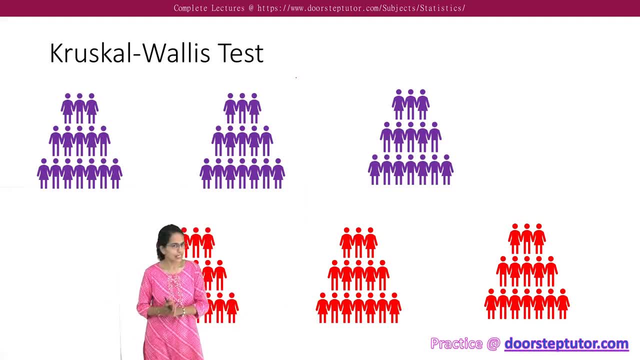 Welcome. In this lecture we would understand one of the very important non-parametric tests, and that is Kruskal-Wallis test. Now, Kruskal-Wallis test is an interesting test Why? Firstly, because it is a non-parametric test, So it is applicable only on the studies where 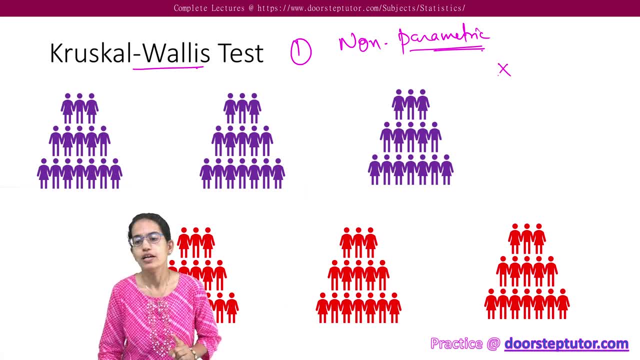 the distribution is not normal. So in the case of distribution being non-normal or not normal, we would apply the concept of Kruskal-Wallis. This Kruskal-Wallis is an equivalent form of ANOVA. What is the major difference? ANOVA is a parametric test. that means it is applied where 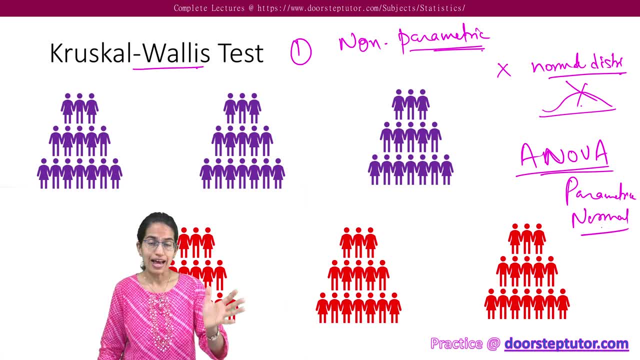 the distribution is normally where the values are normally distributed. However, Kruskal-Wallis is a non-parametric test applied where the values are not normally distributed. In both of the cases, there should be 3.. 3 or more independent samples- Very, very important When we talk about Friedmann test. 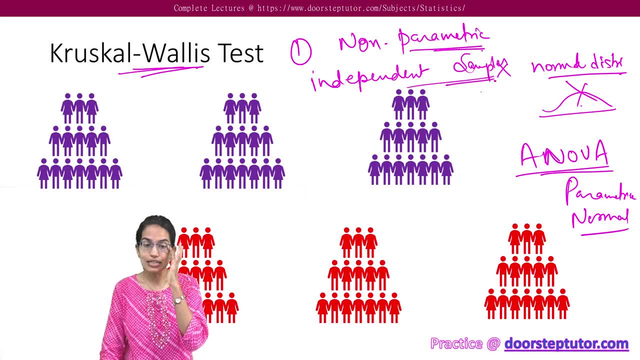 we use dependent samples. However, here the samples are independent, So none of the values in this, this and this match. So when we talk about ANOVA, we take the difference of means. So of this value, what would be the mean value That would be taken Of this value? 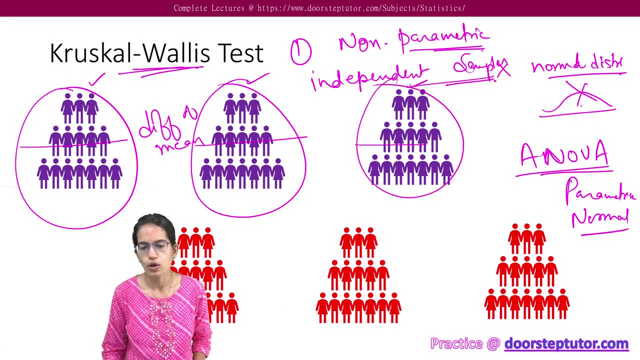 what would be the mean value That would be taken, And the same for all the three groups independently. However, when we are talking about the Kruskal-Wallis test, we assign the ranks. Now these ranks are interesting In Kruskal-Wallis, so Kruskal-Wallis is difference of ranks. 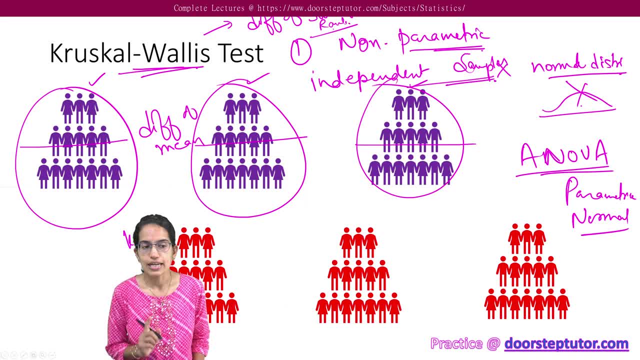 and sum of ranks. right Now, when we assigned the rank in Kruskal-Wallis, what is unique? The smallest value is assigned rank 1.. In contrast to this, when we are talking about Friedman test, highest value is assigned the rank 1. so let's say, within all of these have different values. 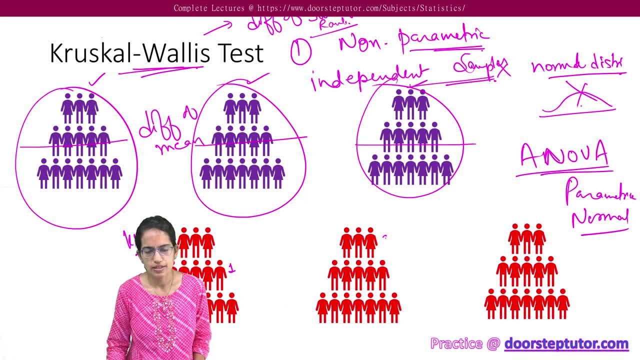 okay, so the smallest value would have rank 1, rank 2, rank 3, then again 4, 5, 6 from this group, only then 7, 8 from this group, 9 from this group, 10 again from this group, and so on and so forth.